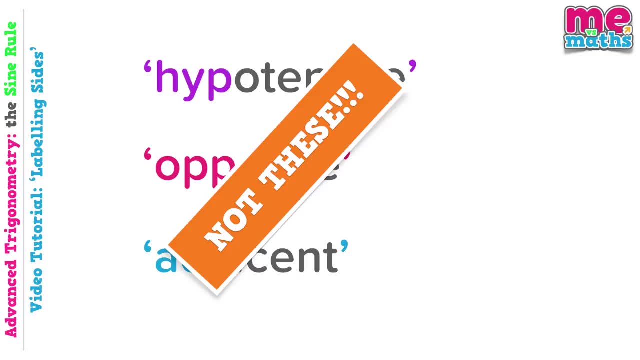 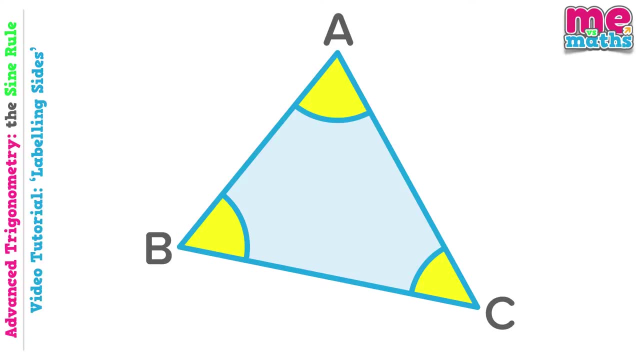 used when dealing with right angled triangles or shapes that can be broken into right angled triangles. Okay, let's look at an example then. You see, here we're starting with a non-right angled triangle, and you can also see that we have some points that have already been labelled A- B. 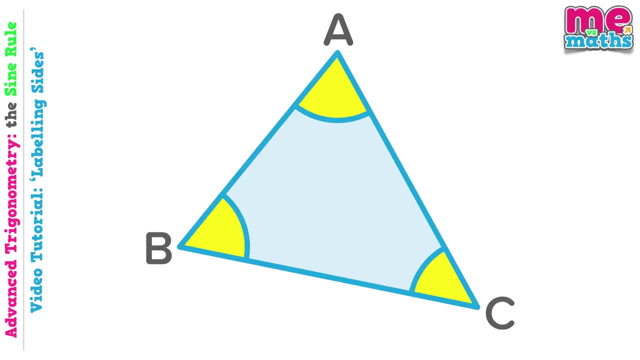 and C. Notice, these are capital letters, which is really important. Now, not only do these capital letters refer to these points, they also refer to the angles at these points. So we'll call this angle, angle A, this angle, angle B and- you've probably guessed it- this angle, angle C. 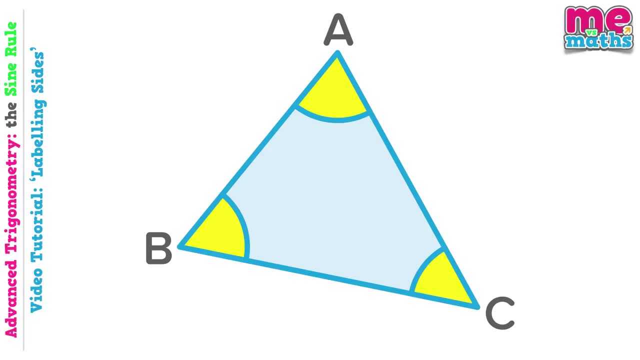 So now we know how the angles are labelled, but how do we label the C angles? We'll start by looking at angle A again. We call the side opposite angle A, side A. Now I know this is a bit confusing. To try and make things clearer, see how we use the lower case letter there for the 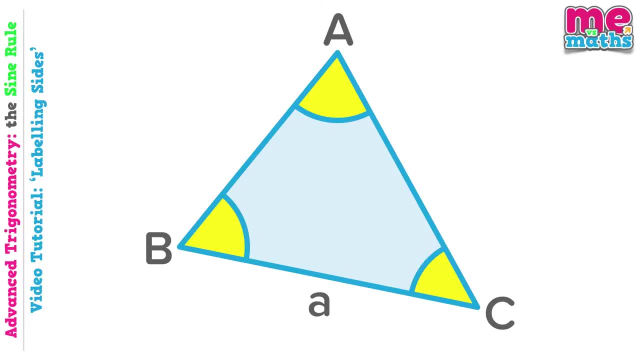 side. So if the side opposite angle A is called side A, you probably won't be surprised to know the side opposite angle B is called side B. Again, notice, the lower case letter is used. And finally, side C will be located opposite angle C. So there we have a fully labelled non-right. 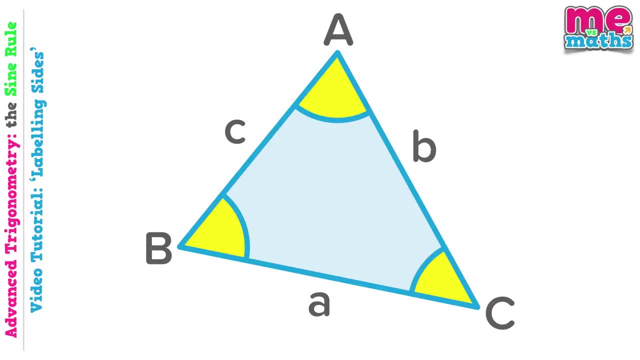 angled triangle, all ready for us to use with either the sine rule or the cosine rule. Let's look at another triangle now and label it up again. Here we're starting from a very different point. We've just been given one side, which is called R. Well, opposite side R, we must have angle. 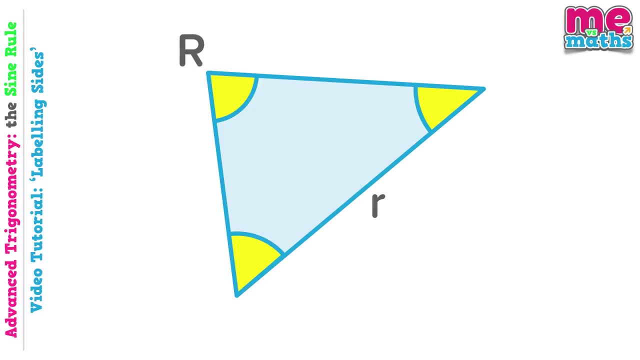 R. Don't forget the capital letter. If we go to this point next, we need to give it a name. Now, we could call it anything, but as we've already got a point R, let's call this point S Opposite angle S. we must. 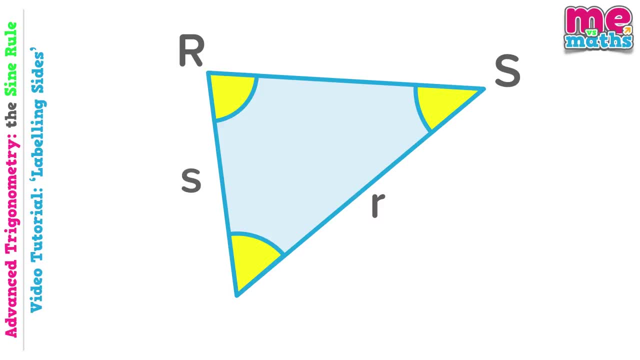 have side S And finally we have this point at the bottom which I'm going to call T, and opposite angle T will be side T. Again, all the sides and angles in this triangle are now in a state where I could use the sine rule or the cosine rule with them, But some people don't like the result. we 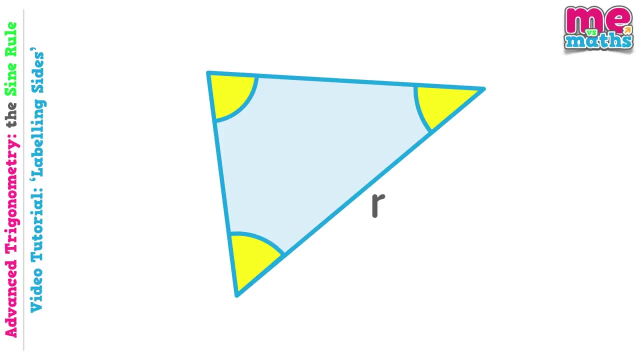 just got, As we're not using A's, B's and C's as we saw in those original formulas, So there is another way we can label this triangle up. If we don't like R, let's just call it A instead. 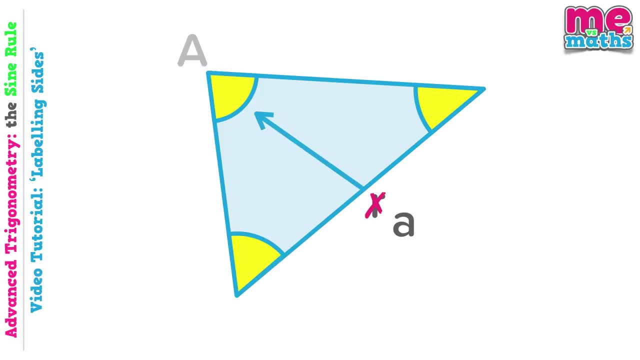 Opposite side A will have angle A. Now let's call this point B. this time Opposite angle is quater, angle B will have side B. and finally, let's have point C and opposite angle C will have side C. So a different way to label up the same triangle, and we could 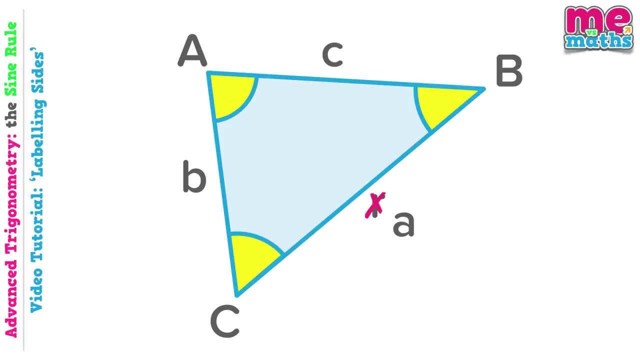 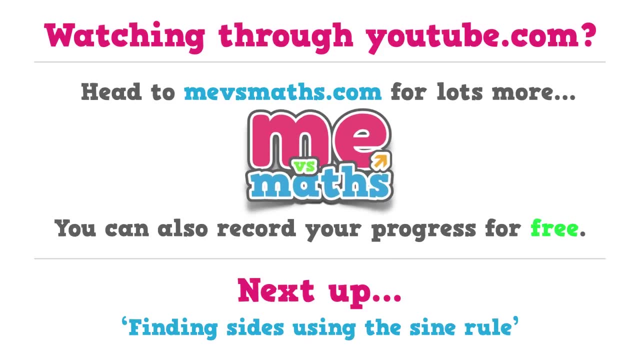 use either of these as a starting point for using the sine rule or the cosine rule. That's all we're going to do in this tutorial today. In the next installment, we'll look at using the sine rule that we glimpsed earlier to find missing sides in triangles. As always, if you're watching through YouTube, please, 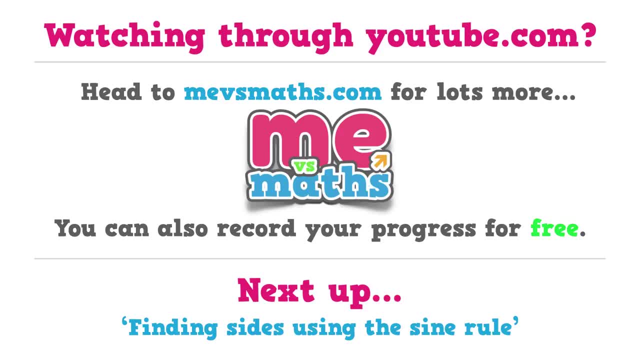 check out the website at mevsmathscom. There are lots more resources available there and you can also record your progress for free. Thanks for watching and I hope to see you again soon. Bye for now.